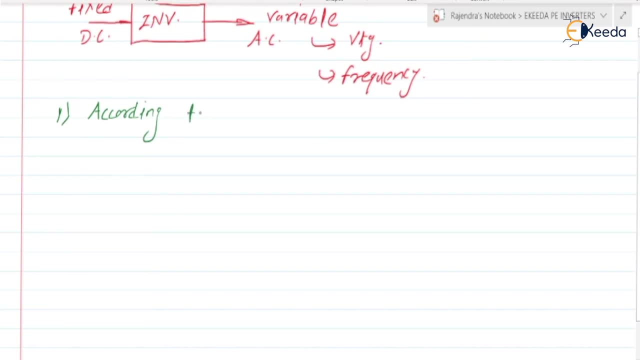 inverters according to nature of input source. according to nature of input source, right, there are two types of the inverters according to this, as first one is the voltage source inverter- voltage source inverter is also known as the VSI okay- and second one is the current source inverter. 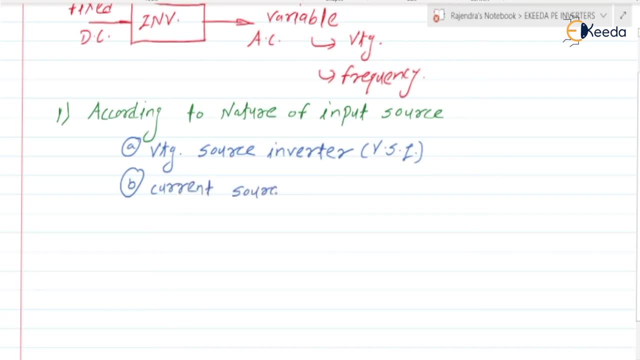 current source inverter. ok, it is known as the CSI. CSI, that is the current source in one thread. one is the voltage source inverter. second, one is the current source inverter. okay, the difference between the tool is in the whole testors inverter, the input mod attached to the 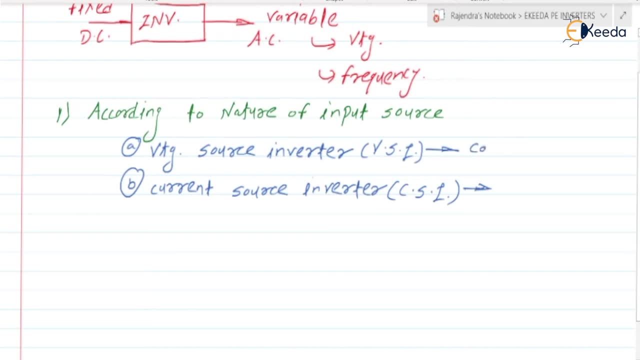 circuitry is constitutional. okay, when here we'll be having the constant input voltage. constant input voltage voltage, right? whereas in the current source inverter, yes, the input current to the circuitry is constant. okay, So here we will be having the constant input current, okay, constant input. 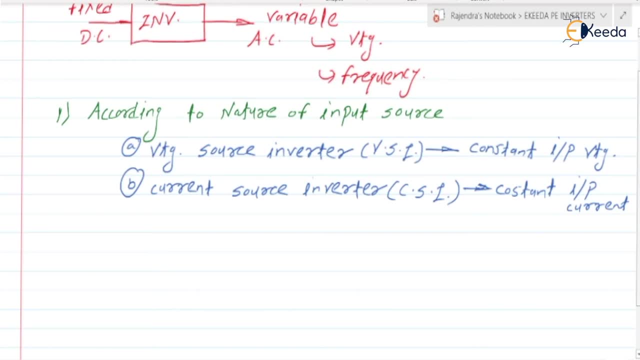 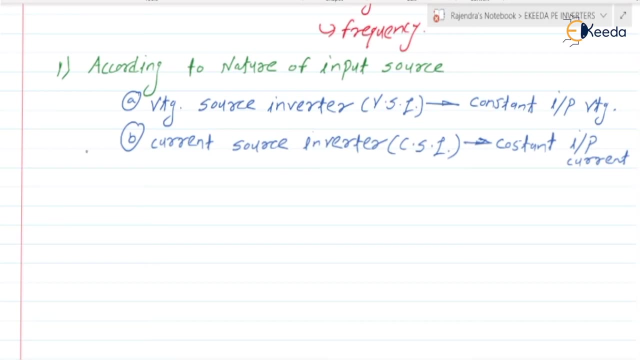 current in the current source: inverter right. So these are the two classifications according to the nature of the input source. Next, the second classification we are having. it is according to the wave shape of output voltage. according to wave shape. according to wave. 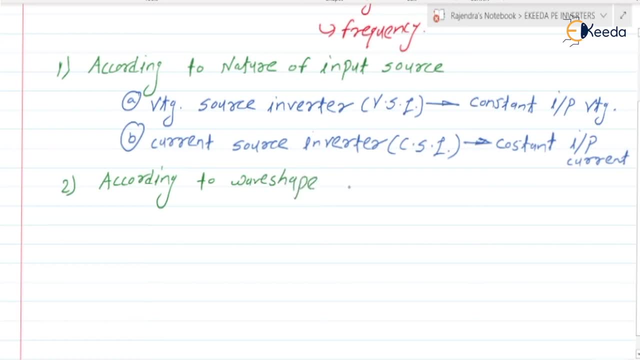 shape of output voltage: output voltage- right. So according to this, or the output voltage- waveform. okay, According to this, we are having the three types. One is the square wave- square wave inverter. second one is the quasi-square wave inverter. quasi-square wave inverter. 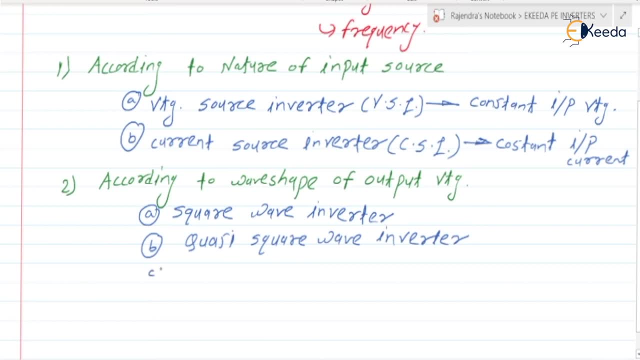 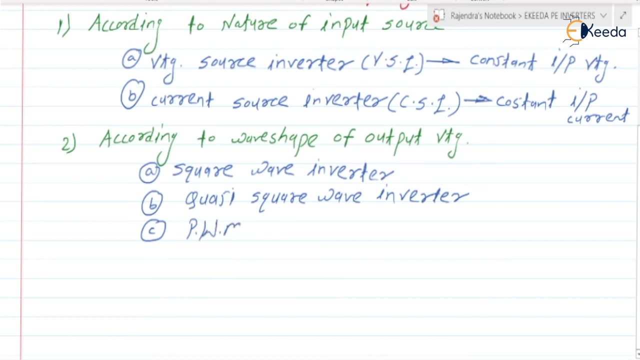 third one is EWM, that is, the pulse width modulated. okay, So in the square wave inverter, the nature of the output voltage, waveform, right, it will be like this: So this is the time t from g0 output voltage. in the nature it will be like this: okay, 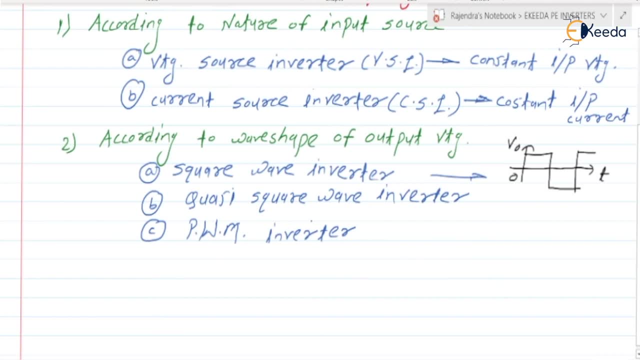 It is a square wave right First in the quasi-square wave. if you check, I am drawing here for the quasi-square wave, the quasi-square wave, the nature of output voltage, waveform. it will be like this: So it is having non-zero value, 0, but in between it is having a zero portion. okay. 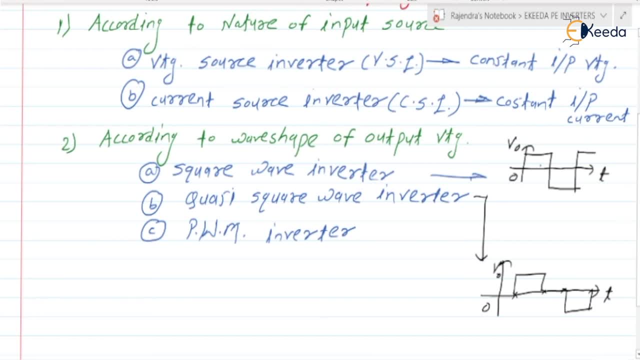 But whereas in the square wave, yes, we will not be having the zero portion in the output voltage, okay, it is a quasi-square wave, okay. Next third one is the PWM inverter. okay, again, depending on the pulse width, modulation. 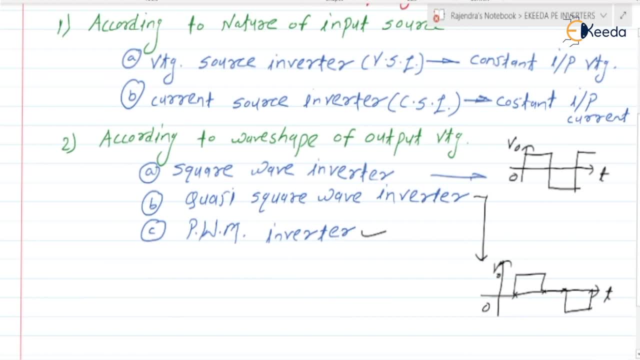 techniques. okay, There are three types That we are going to discuss. Those we are going to discuss, okay, And accordingly, the nature of the output voltage is also changing, okay? Next, the third classification is according to the connections: according to the connections. 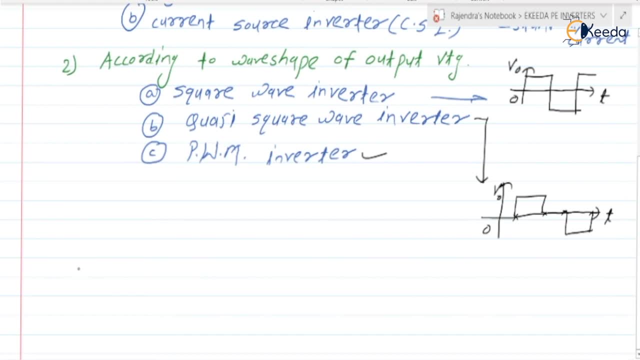 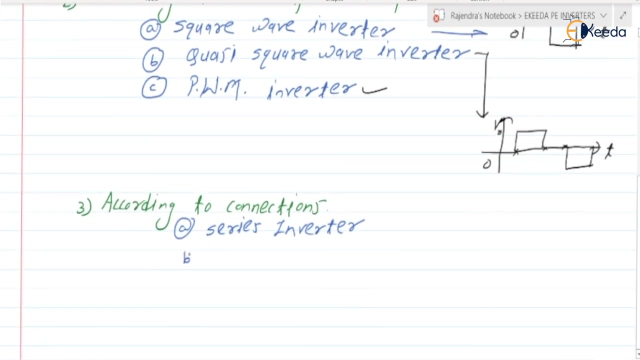 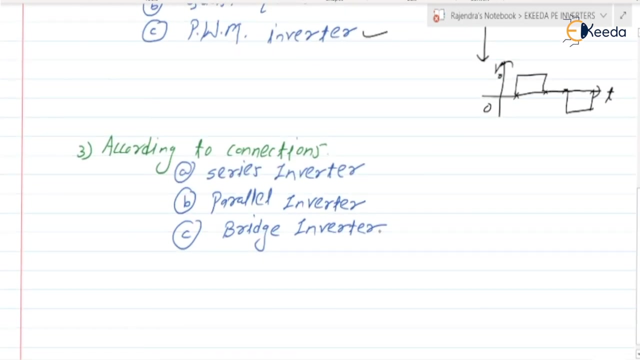 Third one is according to the connections. According to the connections, there are three types of the inverters: First, one series inverter. second, one parallel inverter, parallel. and third, one freeze inverter. Yes, so series inverter, parallel inverter and bridge inverter right.